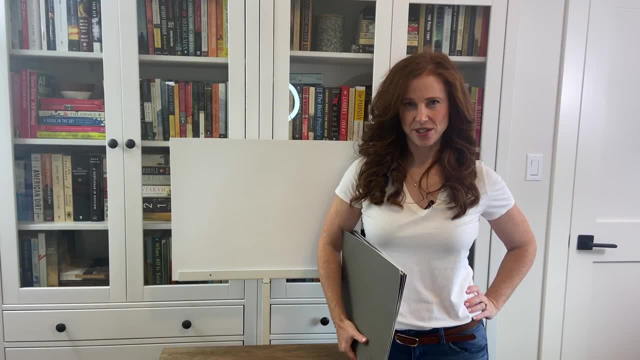 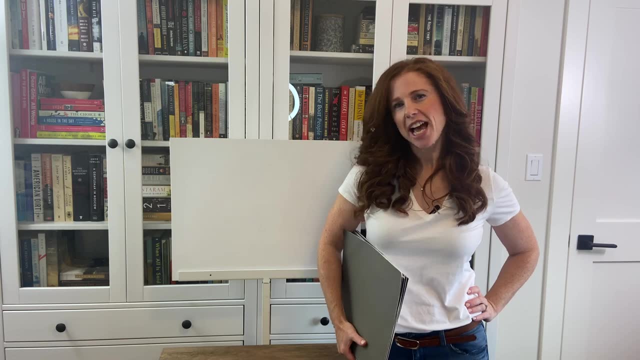 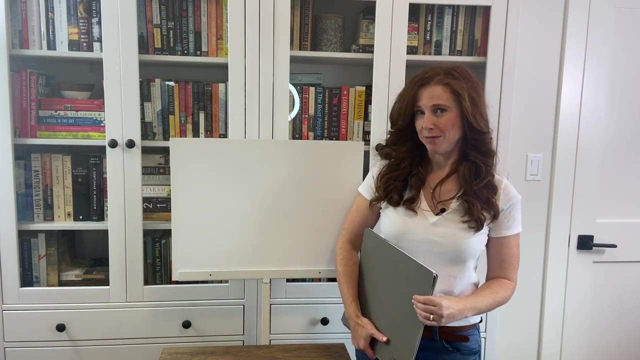 Hey, I'm Kylie of Kylie M Interiors online paint colour consultant and e-design expert. Today, we're taking another look at colours for your kitchen cabinets: island, bathroom, vanity, front door, feature wall- with a specific focus on cabinets, though, and we're going to be looking at 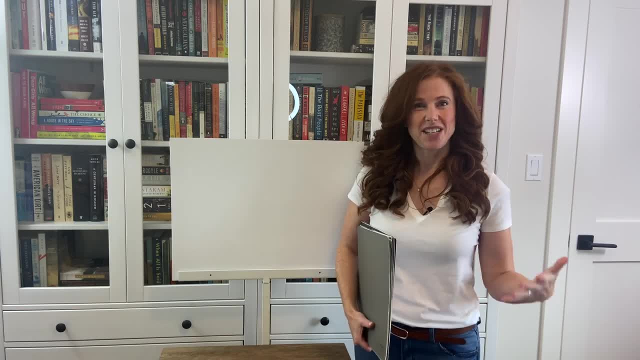 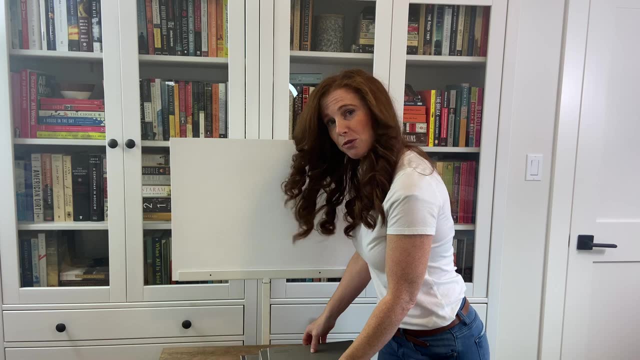 greys today. You can also check out my other reviews on navy blues, and I'll be adding more every week. So we're going to look at grey and black paint colours from Sherwin-Williams and Benjamin Moore. You might want to have a pad of paper and a pen ready so you can make notes on. 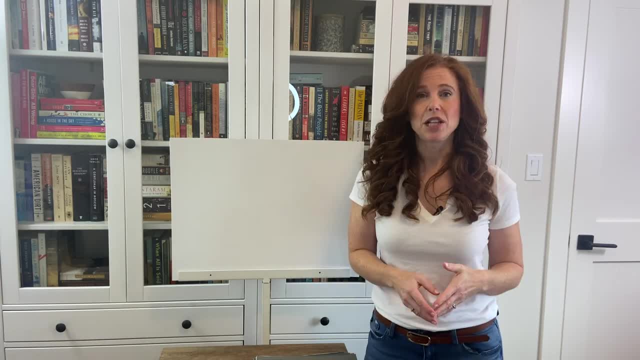 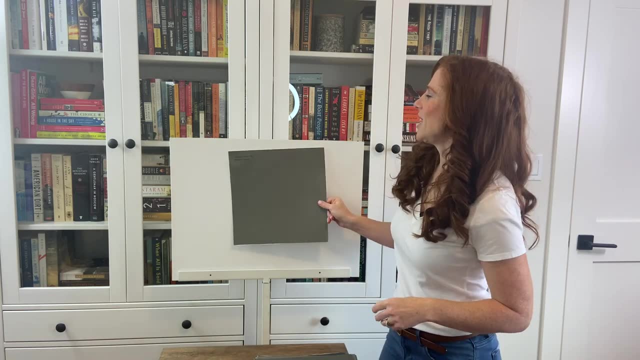 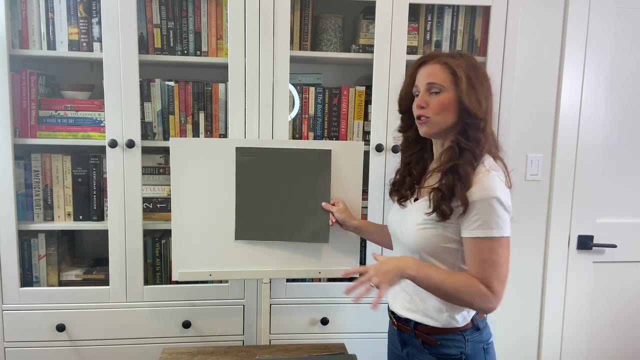 your favourites, And for a lot of these you will find their colour reviews on my blog or independent colour videos. So let's get started. Benjamin Moore, Chelsea Grey- Super popular grey- It's been kicking it for a long time. It's a medium depth grey, so it doesn't have as much visual weight. 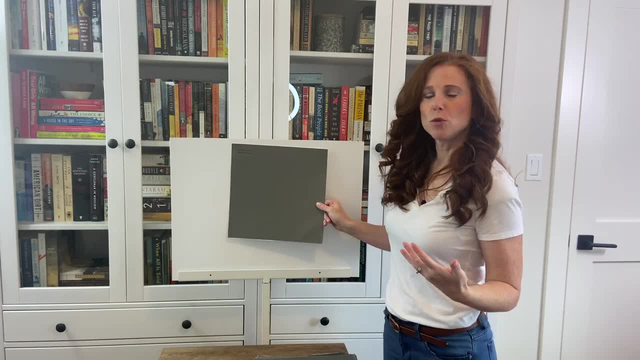 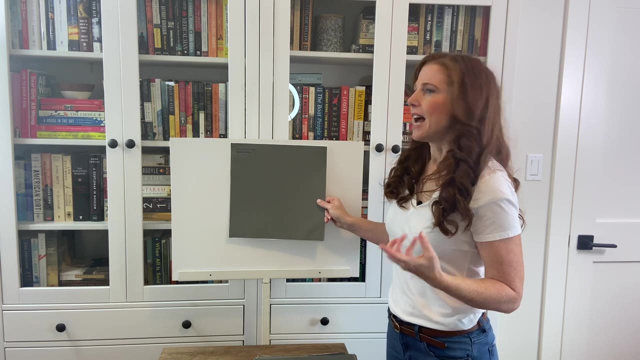 as some of these Super blackish and is super suitable for an entire kitchen without feeling weighed down. Now, you wouldn't notice it, but Chelsea Grey is very slightly warm, with a little green undertone to it. The green doesn't always show up, but you have to be aware of it. So if you had a countertop with a 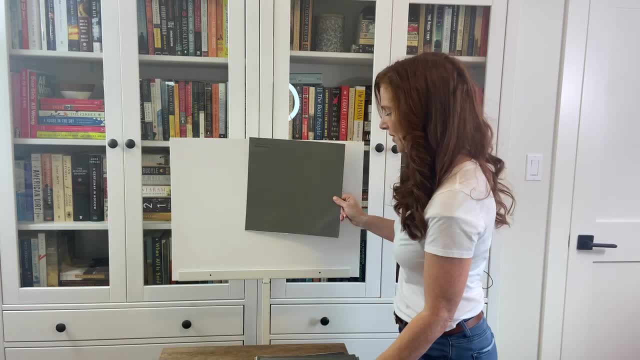 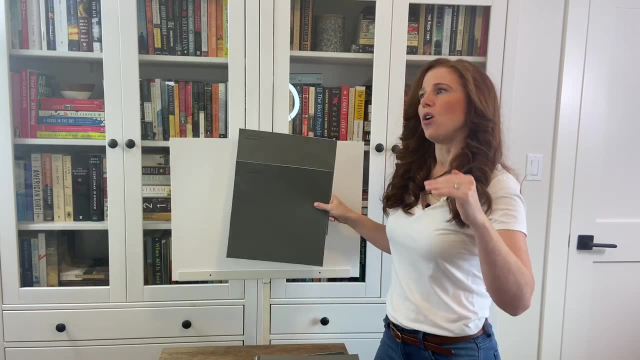 grey, with a bit more of a purple undertone. they're going to clash. Let's move down to Benjamin Moore, Amherst Grey, These three that we're going to look at here. they're all above each other and below each other in the fan deck. 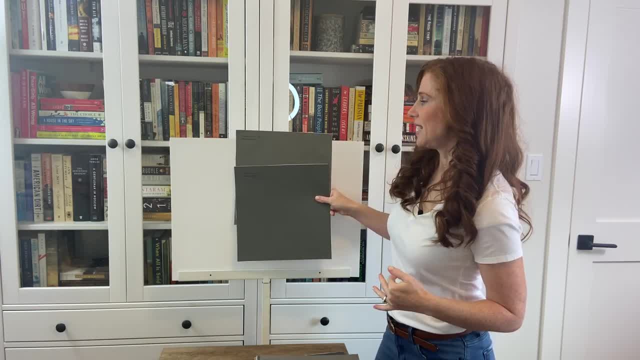 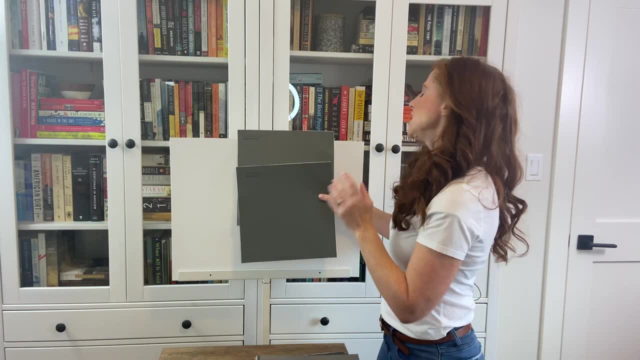 A lot of people refer to them at the same time. Amherst Grey is a little bit darker. I believe it's LRV is. I'm going to say it's 19, but don't quote me on that. So again, it's a soft grey. I'm hard. 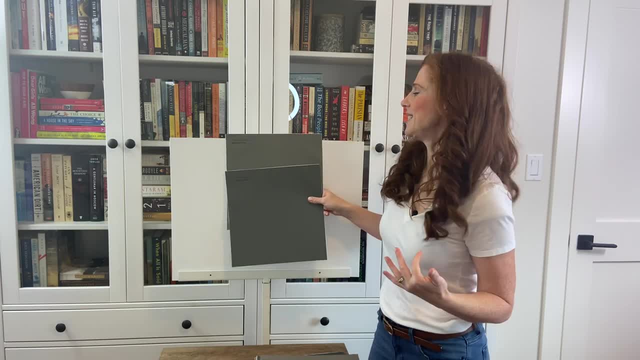 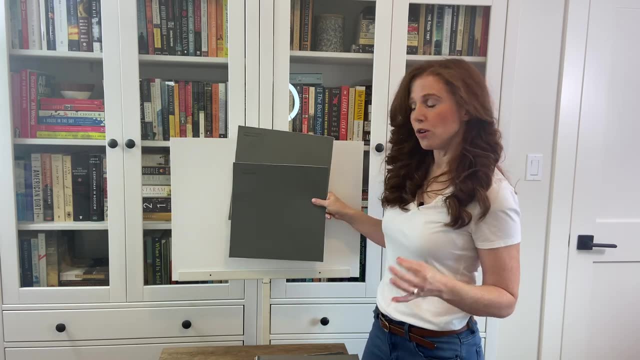 pressed to call these warm greys, because there are legit warm greys out there. They're just not icy cold, They're just soft, with that little bit of a green undertone. Amherst Grey has a wink more green than Chelsea. Again, it can fall back a bit, but don't expect it to. 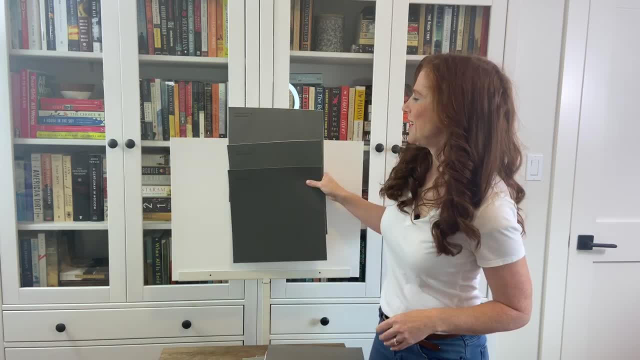 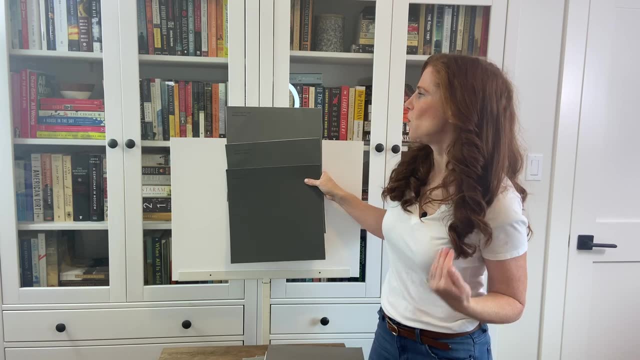 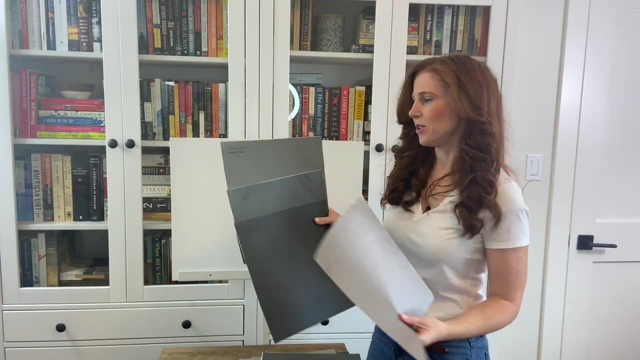 And lastly, in that series, Candle Charcoal: The darkest, super striking, awesome. on an island front door. These colours can do so many things. Now I was saying how these are kind of soft and considered warm greys. We're going to see a warm grey There. we go right. So this is Benjamin. 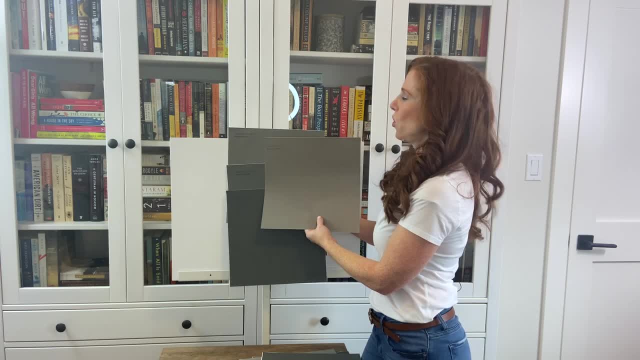 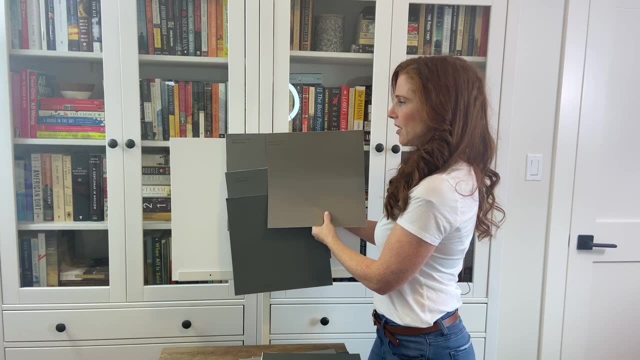 Moore Metropolis. Metropolis is a typical warm grey, has a soft purple undertone and that undertone might help you see that bit of grey. It's a bit of a green undertone but it's a bit of a green in the other options there. If you have a home from the 90s, say 2000s, that has granite and 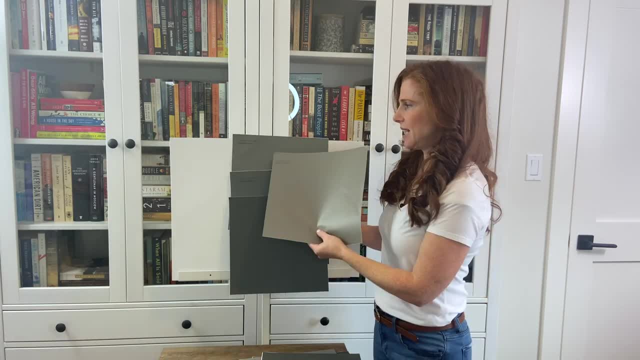 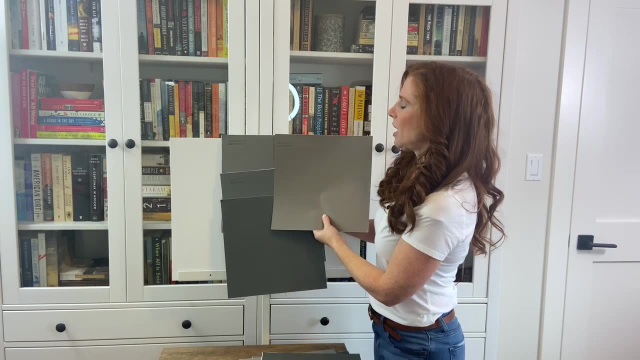 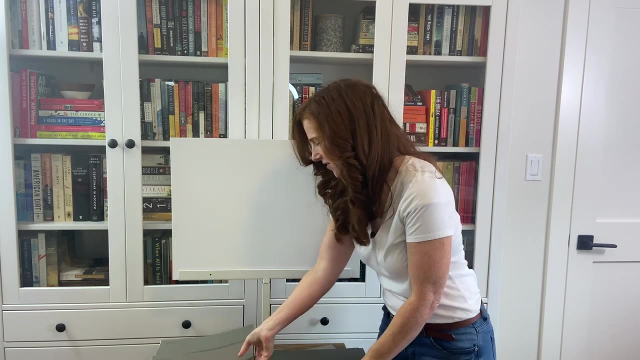 some of those beige tiles. Metropolis is often better than these because those products usually have a softer, warmer, grey or kind of taupe approach to them, So that's why it's a better fit. So let's move on to a couple of my faves. We're going to look at Sherwin-Williams now- Dovetail. 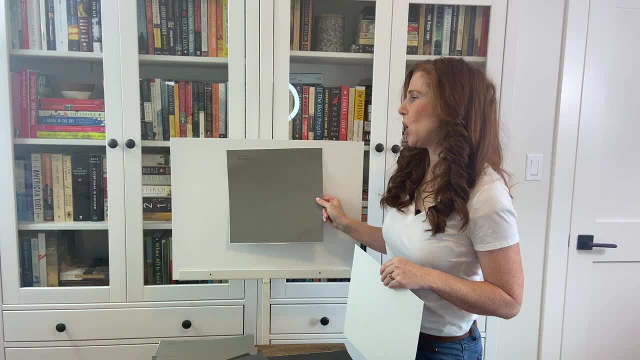 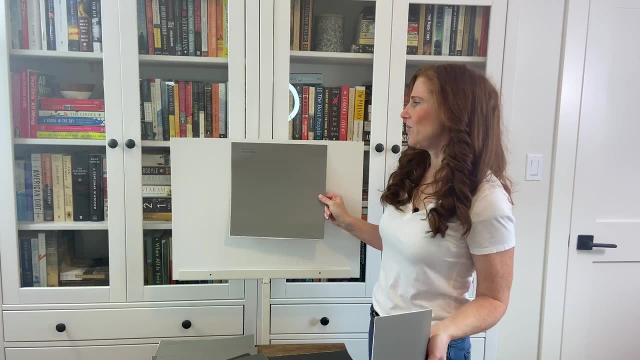 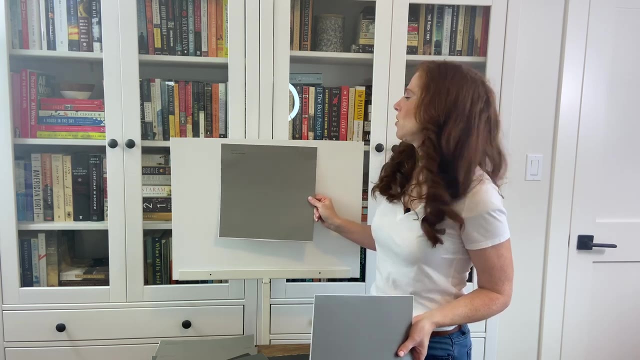 So up there with Benjamin Moore, Chelsea Grey, it's one of the most popular. It's another depth that you could paint your entire kitchen and not even blink an eye. Island, bathroom vanity, whatever you like. Now, Dovetail is a slightly warm grey. It favours a minor purple undertone. 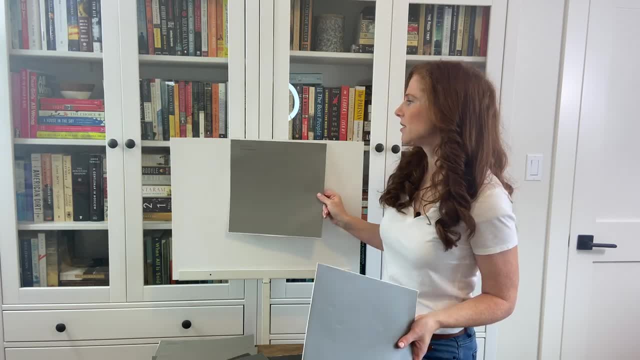 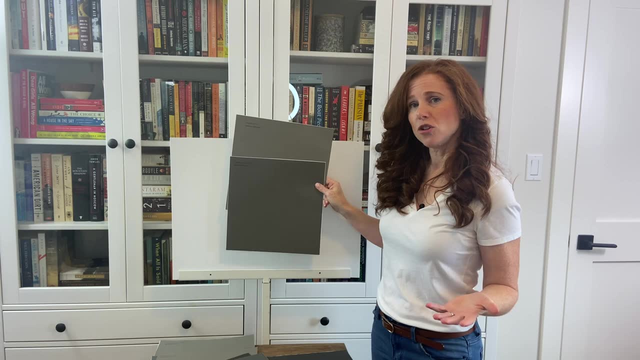 and there's a whisper of green in there, but you'd hardly know it. We're also going to look at the slightly darker version, Gauntlet Grey. You're less likely to see an entire kitchen painted Gauntlet Grey because it has that more depth. So if you're going to paint a whole kitchen, it's a bit of a green undertone. So let's move on to the next fave, Dovetail. So up there with Benjamin Moore, Chelsea Grey, it's one of the most popular. It's another depth that you could paint your. 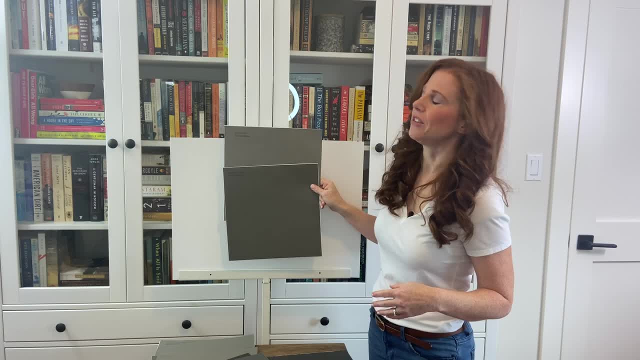 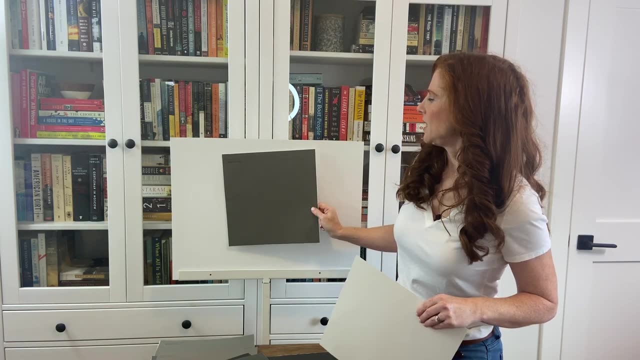 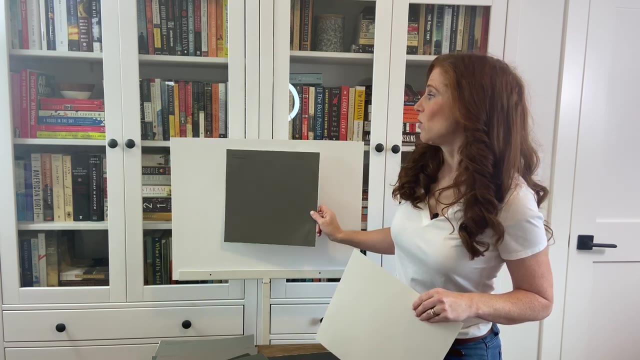 depth to it. great, so great. for an island, though, love it. so again, let's look at that so you can see the light's going to reflect off it, and that's because your cabinet samples should be done in a satin finish, because that will be the finish on your cabinets and you can see how satin finish. 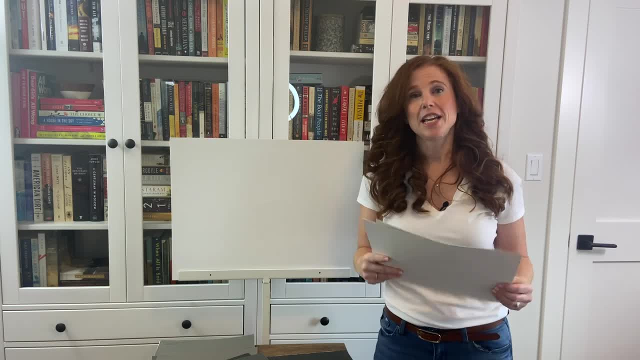 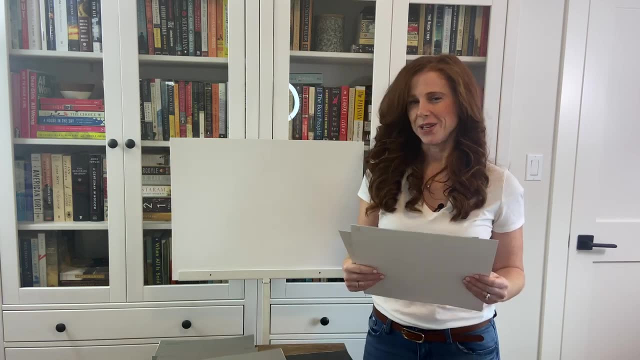 reflects light, so even colors that are pretty dark can look brighter when light hits them. i'm going to show you a few now that have a bit more undertone and warmth. i kind of snuck them in. we have sherwin-williams grizzle gray- okay, this one doesn't have more warmth. 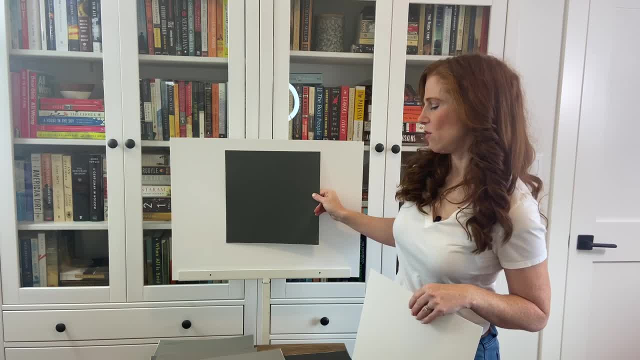 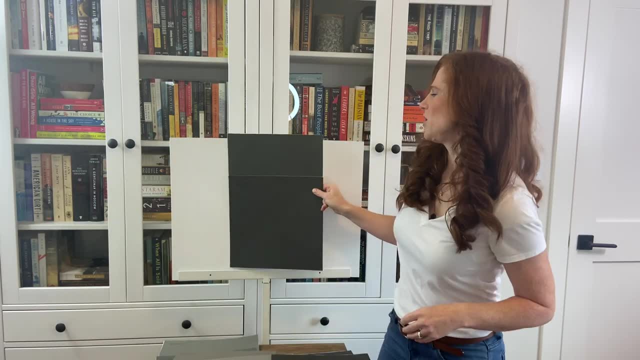 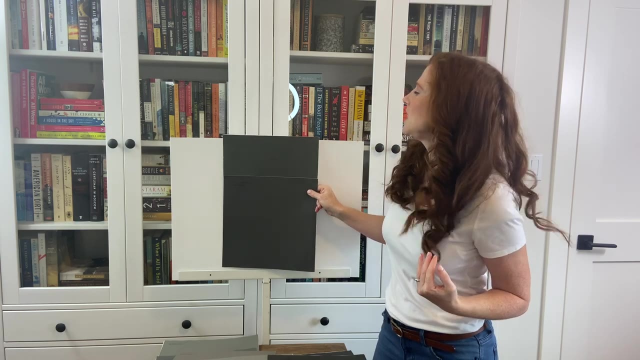 has more undertone. so grizzle gray is a gray with a good green undertone. let's grab kendall, yeah, so kendall charcoal, which we looked at, that might help, you see, that shift that little bit more green in it. i'm obsessed with grizzle gray but it's not everyone's cup of tea. love it. 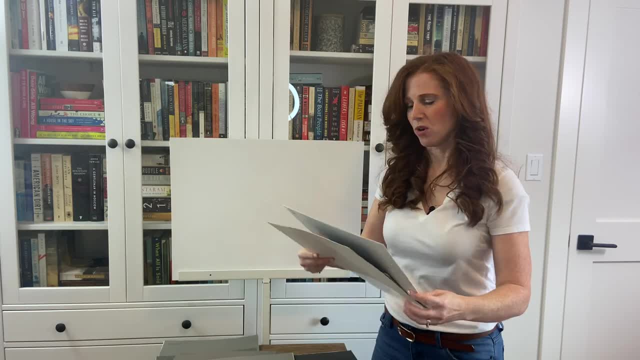 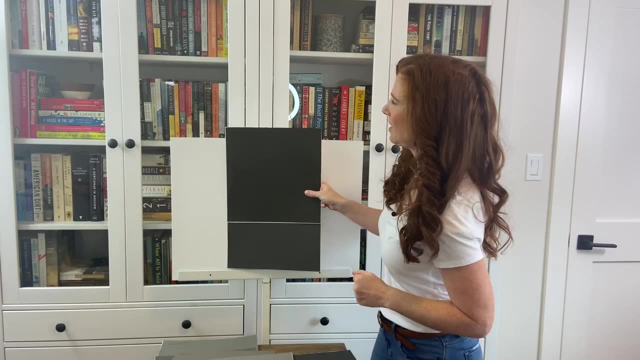 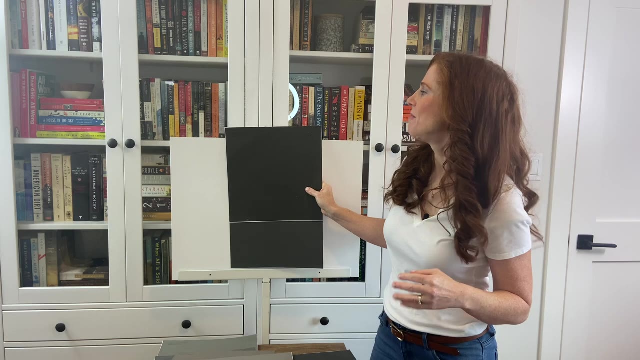 though, and urbane bronze. so this is actually a dark grayish with a green undertone. you can see there's more warmth compared to kendall. this is actually the color of the year. i have it on my island and on my stair railings if you go to my, if you're curious, go to my blog, find my projects and go. 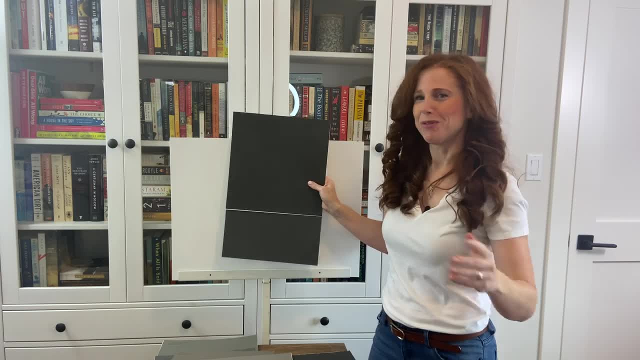 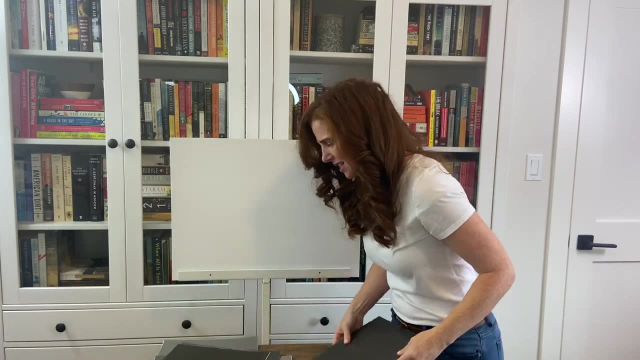 into my homes, not not that i have multiple homes, but find my home section, and in our newest home you'll see urbane bronze in action. but let's move back to what you actually came for, which are the grays. let's move to peppercorn. so peppercorn. 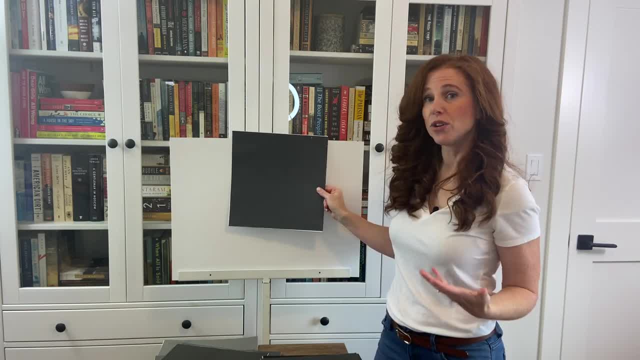 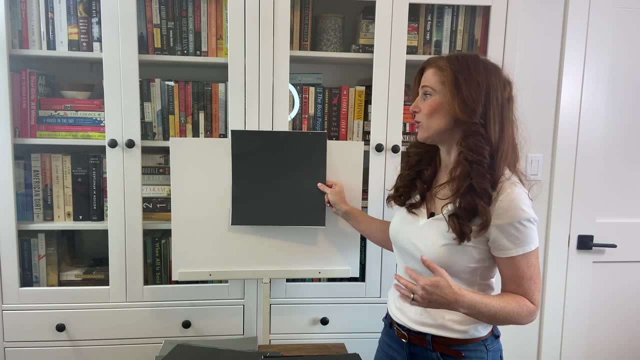 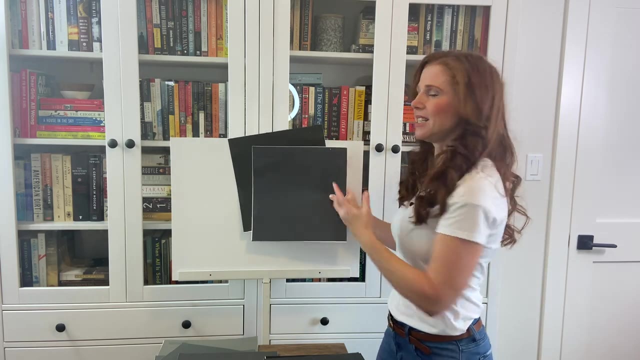 it is a charcoal gray but it has considerably stronger undertone to it. it casts a bit of a blue purple. once in a blue moon you get a wink of green, but don't expect it. let's compare it to- oh yeah, well, urbane bronze, which we just looked at. that might help you see that degree of undertone. 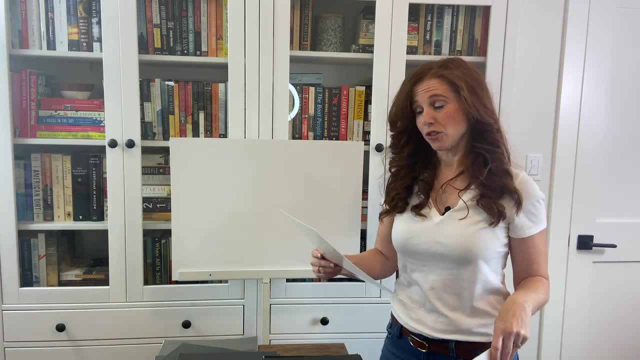 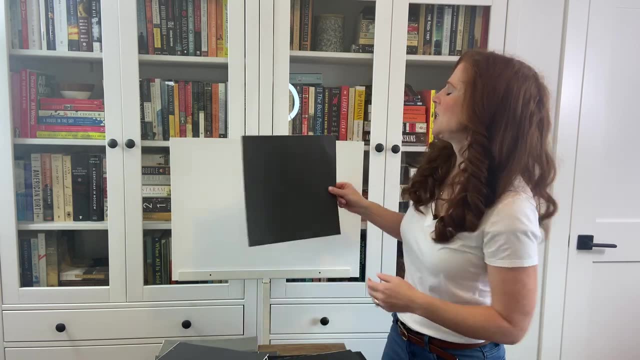 in there. it's a great way if you want a gray look, but not a flatter gray. you want a little bit of an undertones. this one is a grays and this one is a toned-down orange. bit more interest and personality. Iron Mountain from Benjamin Moore: Simple, neutral, darker. 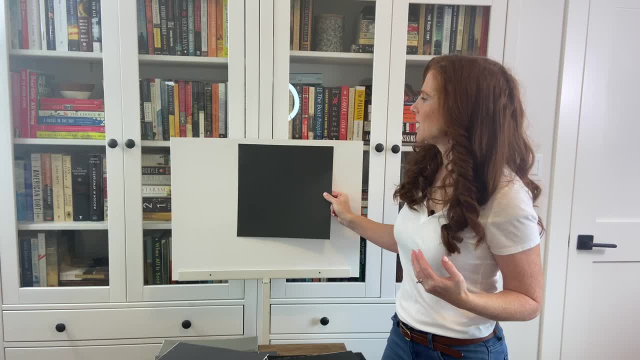 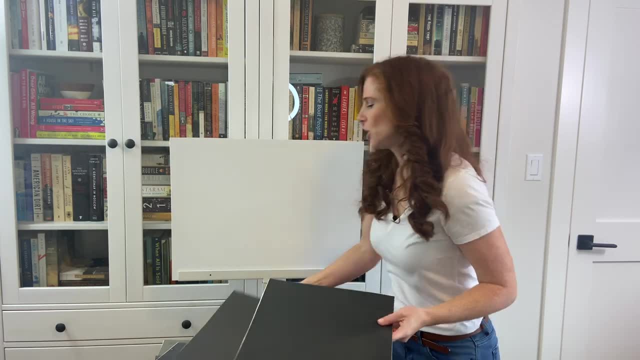 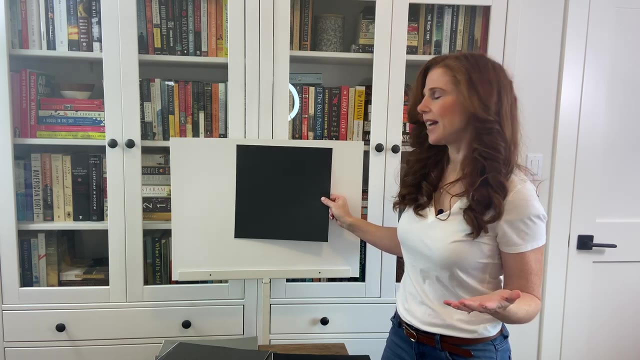 kind of sultry. Most people wouldn't paint their whole kitchen this color, but if you're feeling brave you can fill your boots. See, we're getting darker and darker. Sherwin-Williams Iron Ore. Now this is a soft black paint color, So it is in the black range but it has a little bit higher LRV. 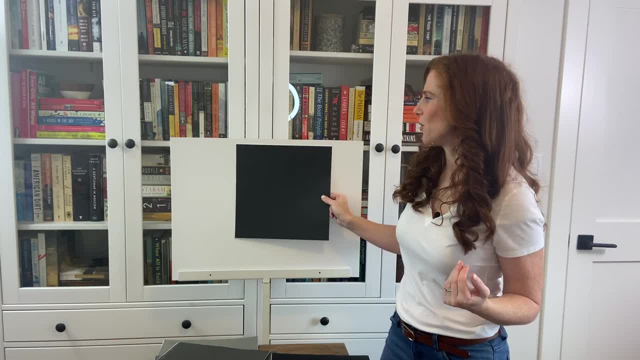 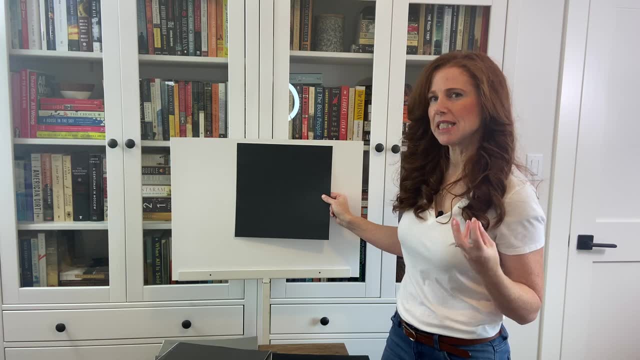 which means it can also pick up that little bit more undertone. It's a sneaky one. I've seen it grab a little wink of green. I've also seen it pick up a funny blue, like an almost slate blue. So you do have to watch it to see it see if it connects with your products, Make sure you see it. 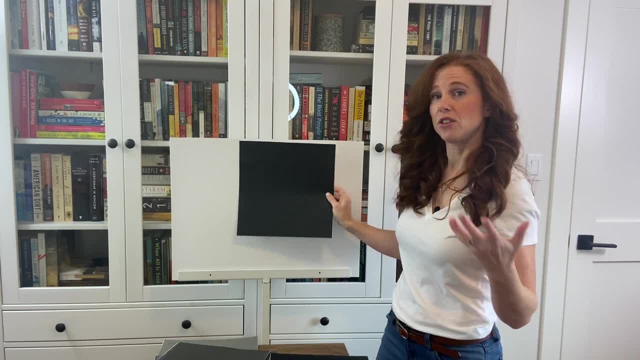 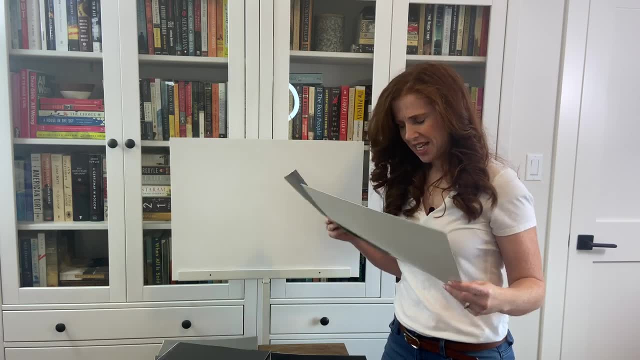 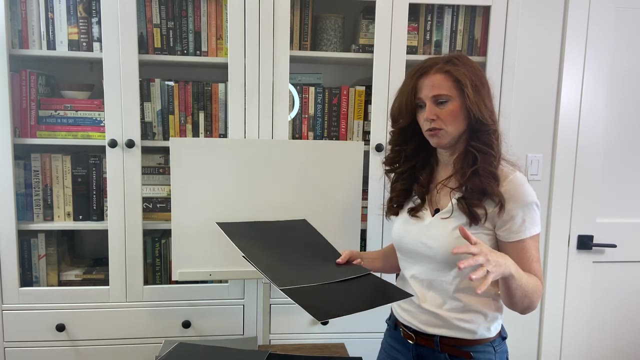 in the light so that you can see how it shifts if the color comes up on you And that might look black. but now we will look at legit black. Which one is this? This is Benjamin Moore: black, like literally black. If you like it, you want to find it, you need the number, which is 21-32-10.. Because if you tell, 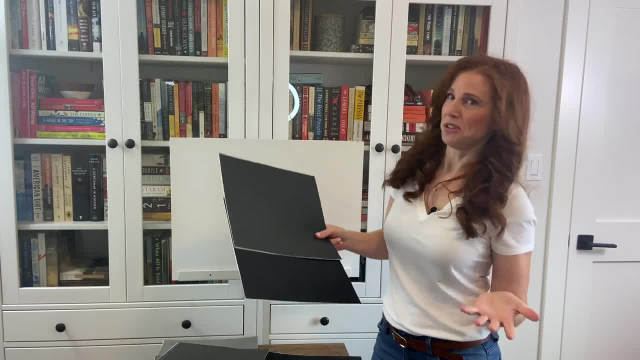 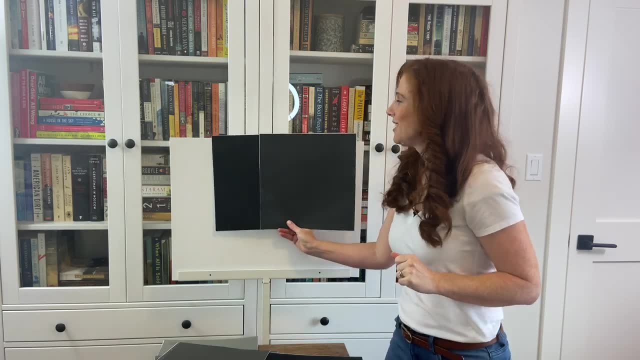 them you want. you go to the store and say I would like Benjamin Moore black. they're going to say: which black do you want? Which is not helpful. So you need 21-32-10 if you like this guy. So